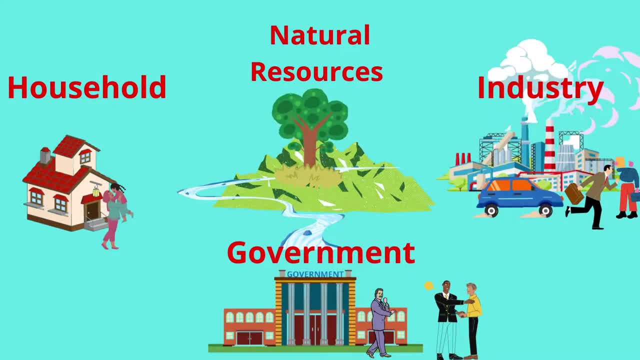 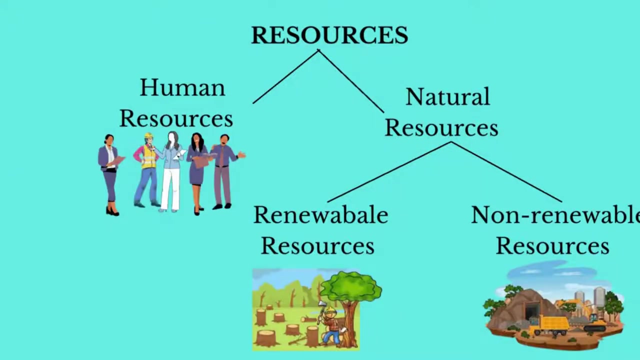 These components include households, industry or economic activities, the government and resources. These components function together to ensure that people's economic needs are satisfied by available resources through the exchange of money. Resources can be broadly divided into human and natural resources. Human resources refer to people, along with their knowledge, skills, talents and abilities. 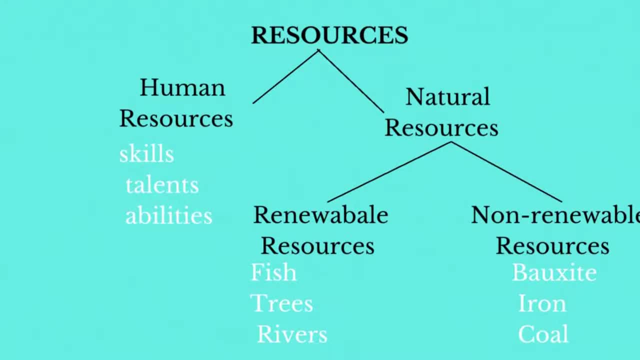 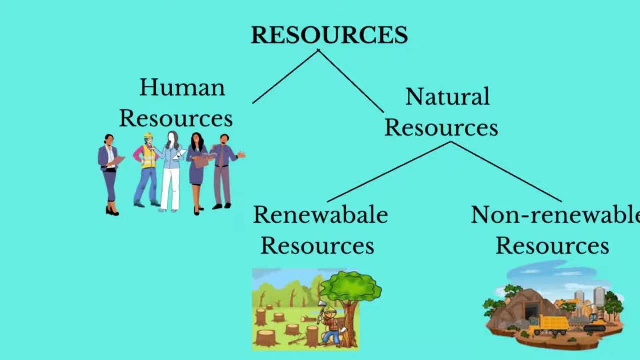 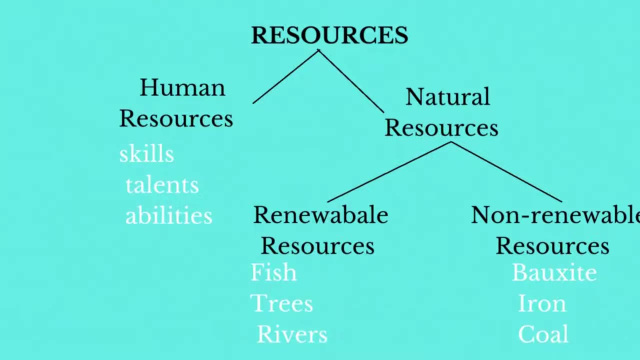 Natural resources are features of the environment used by people to satisfy their wants and needs. Natural resources such as crops, fish, trees and other natural resources are used to fulfill their own 준비 needs. We have a wide list here to recommend our options. 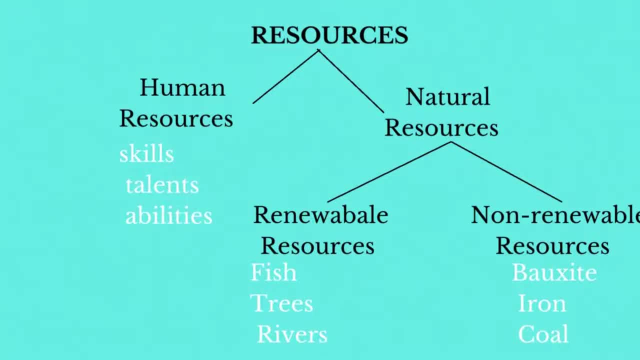 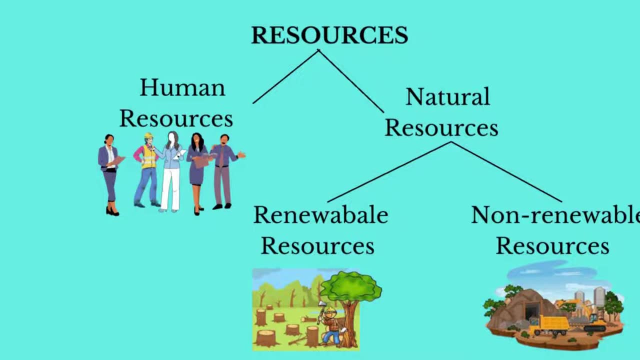 Energybrushes质 assistir器 andolf tree kavanolyakas are a variety of natural resources. I'm going to talk briefly about the various sources track it comes with, including crude oil, waste resources, the sitar cutting technology. there's also some that are marked here which represent contemporary and old, and some that are 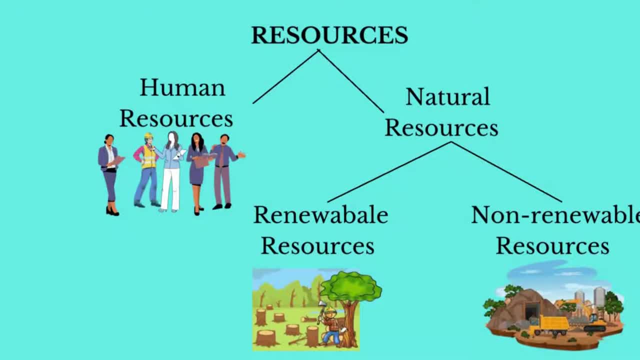 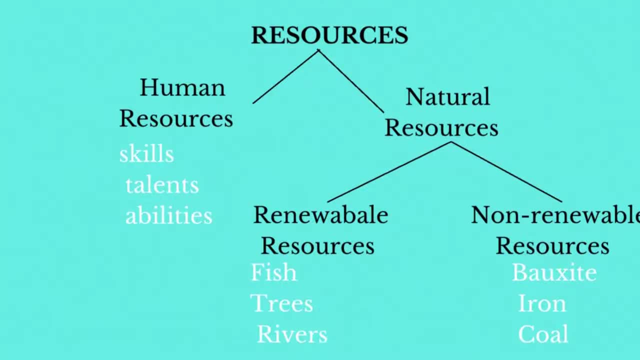 now 가지able resources. These are the kinds of materials that can be used or toblick and PGOs that provide the right比如, Non-renewable resources include fuels such as oil, coal and natural gas, as well as minerals such as iron and bauxite. 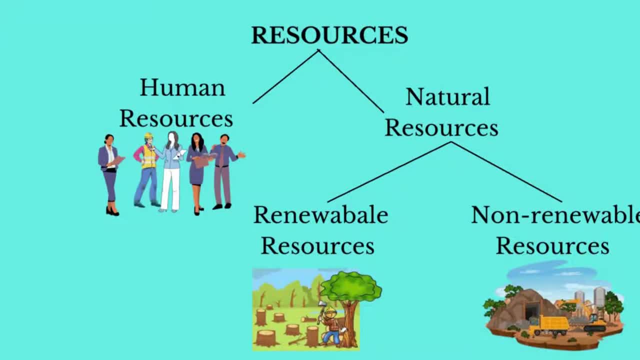 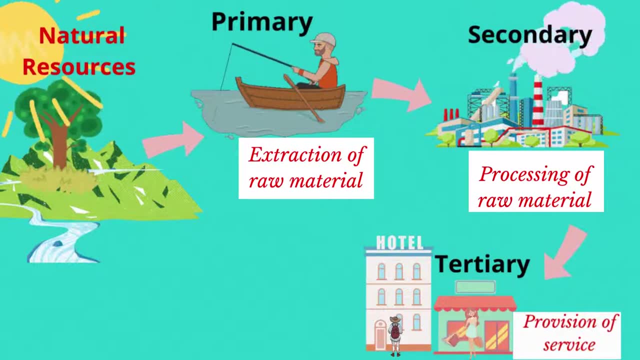 Non-renewable resources take millions of years to form. Now, natural resources are extracted and or harvested by primary industries, which include fishing, mining, farming and so forth. These industries produce raw materials. Some raw materials can be consumed in their natural state, while others will need to be altered or processed in order to be useful. 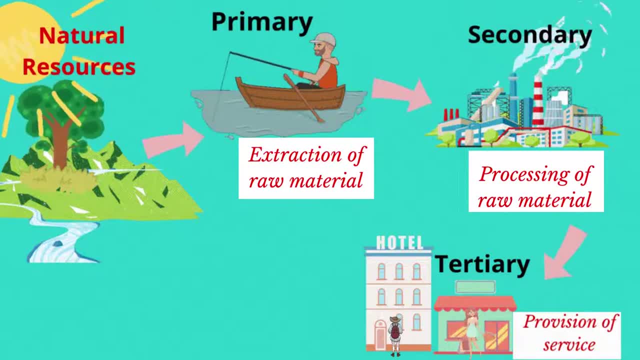 This processing of raw material is. This processing of raw material is carried out by secondary industries. Secondary industries add value to the raw material. They include manufacturing industries and construction industries. Both primary and secondary industries create tangible products or goods. Tertiary industries, on the other hand, do not involve 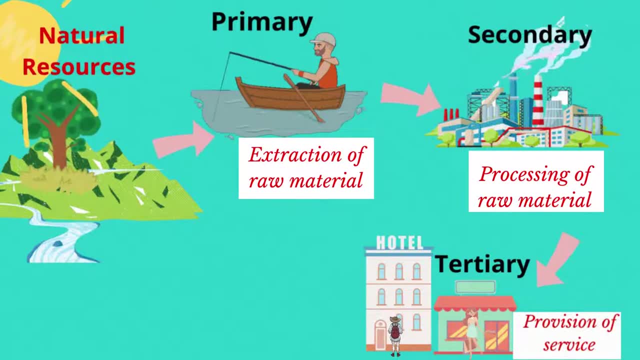 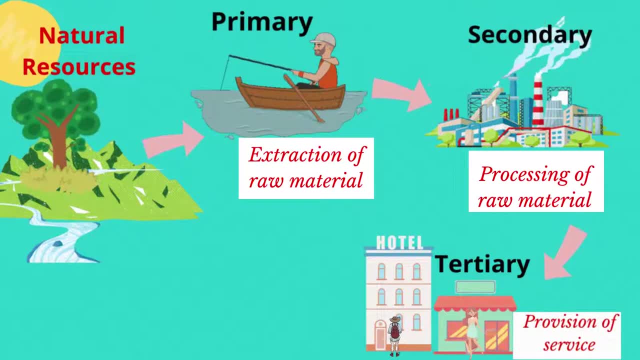 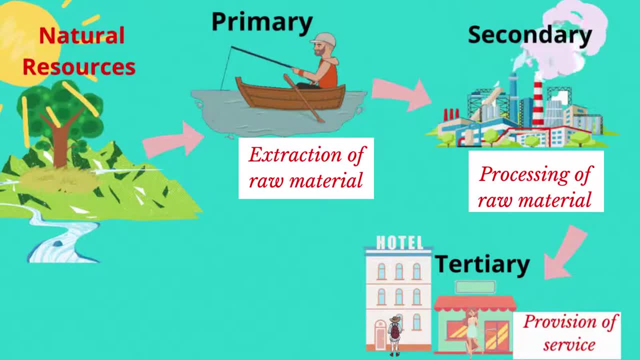 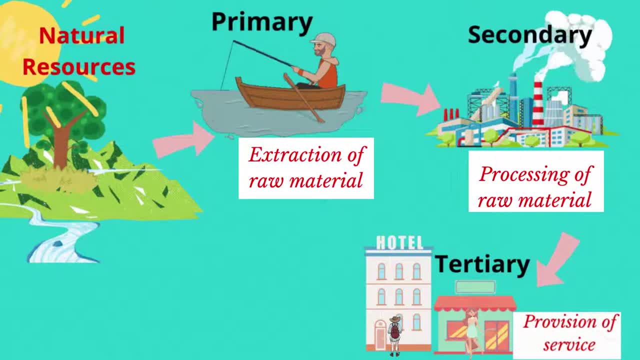 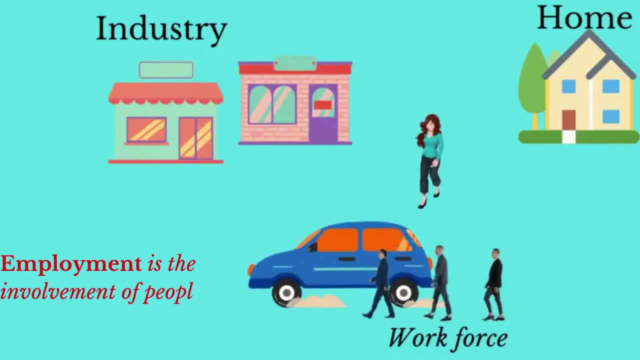 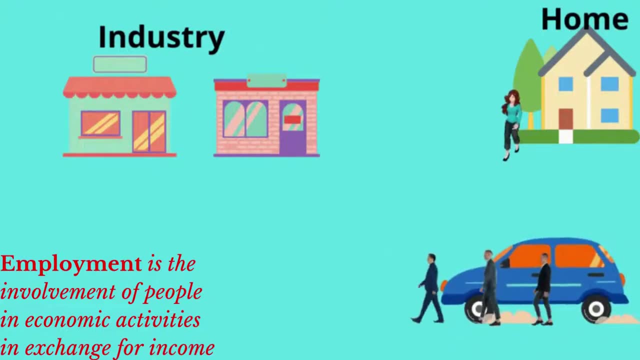 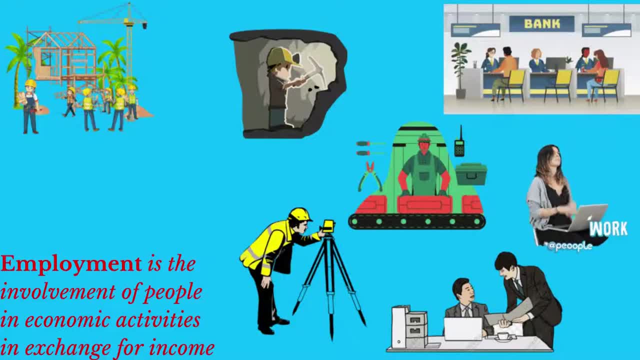 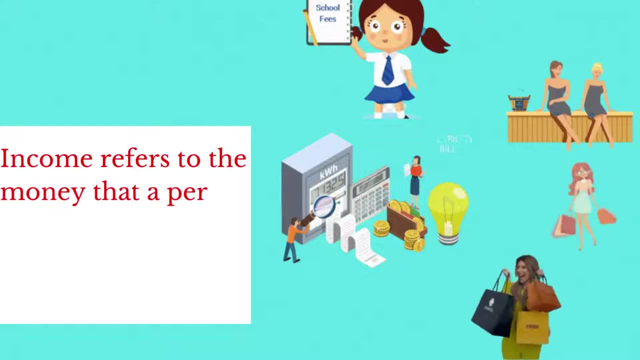 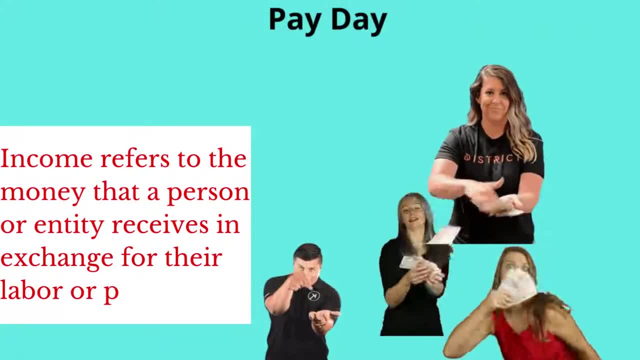 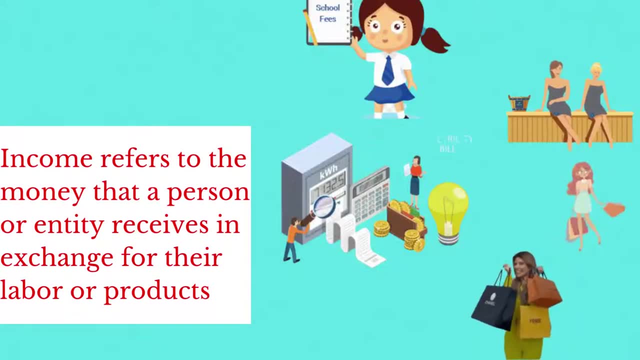 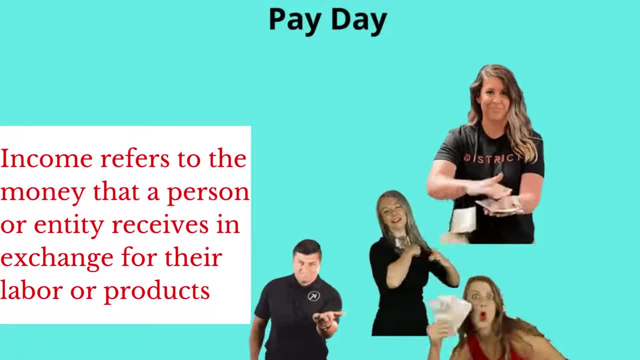 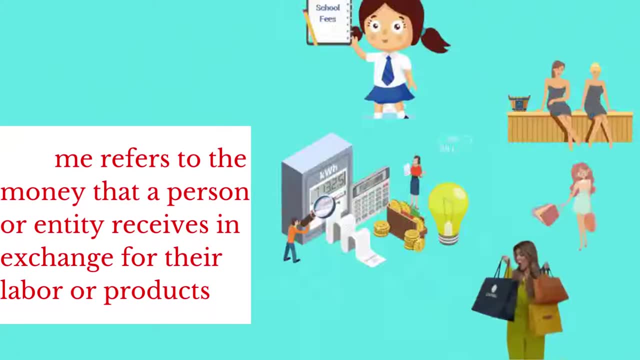 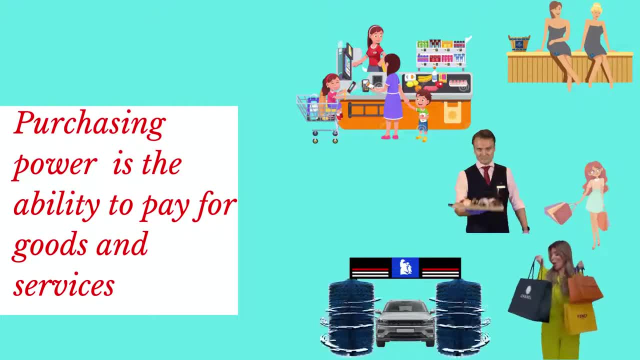 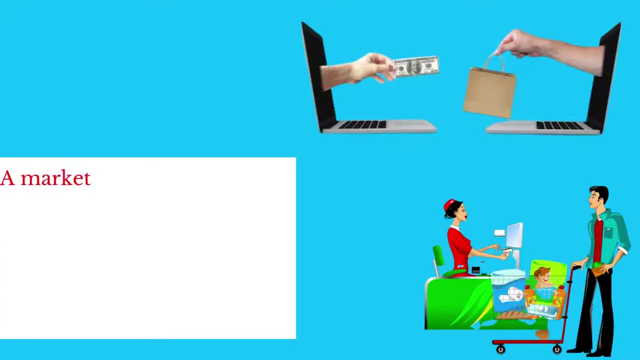 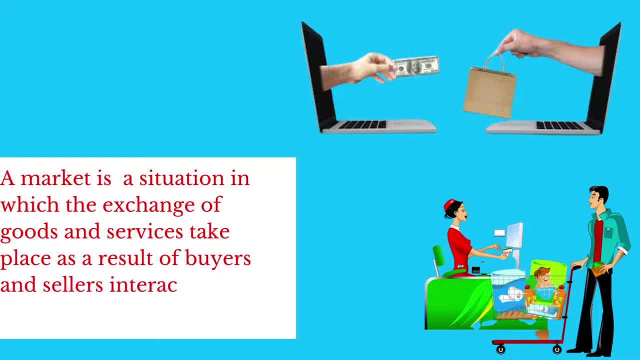 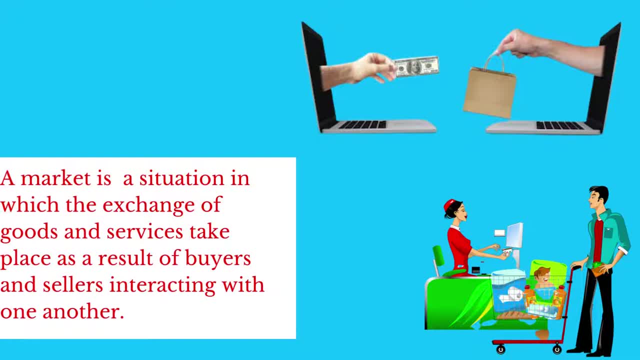 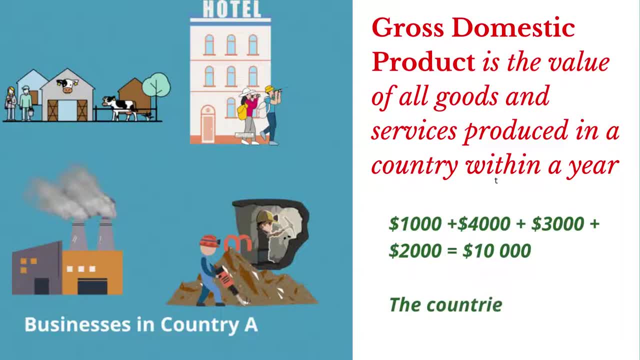 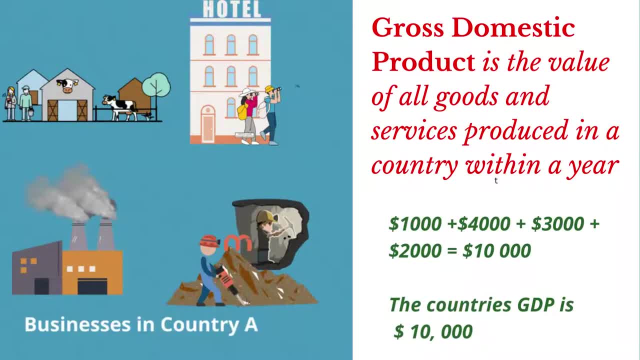 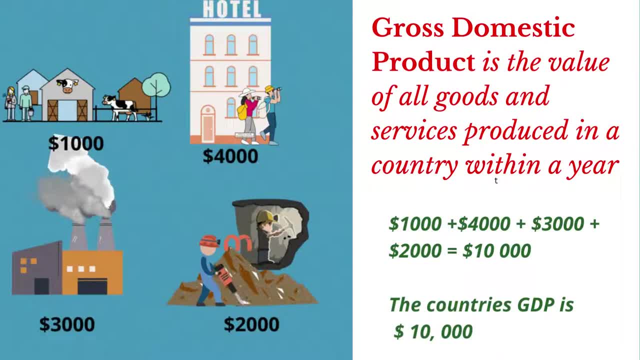 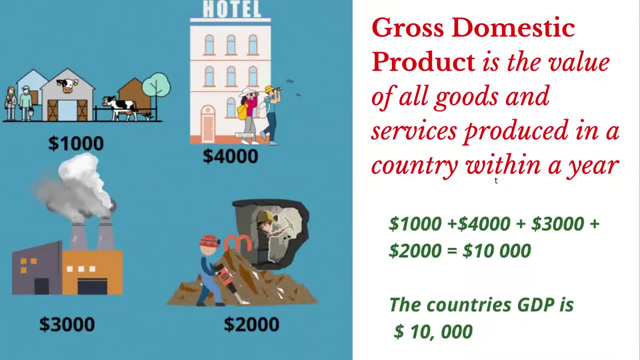 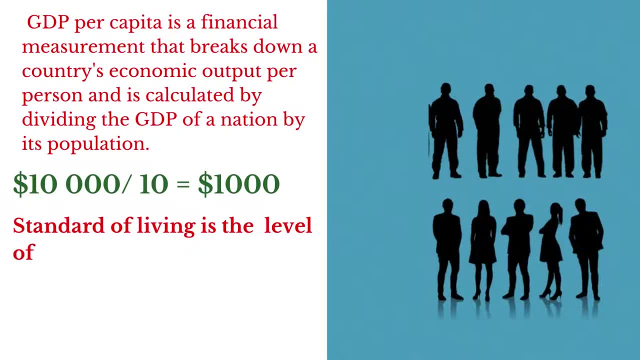 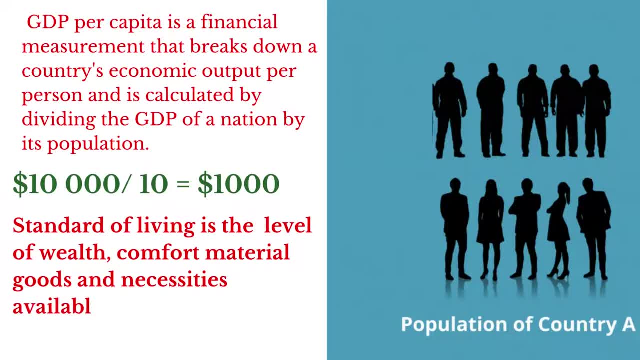 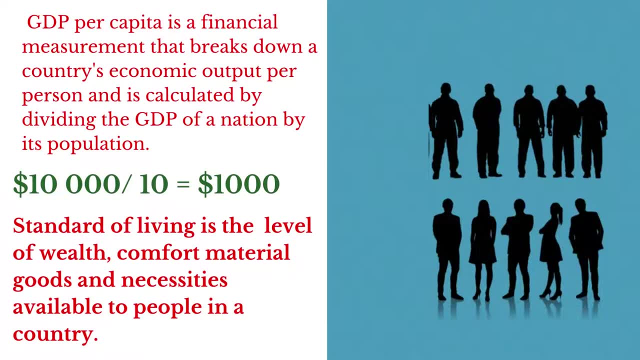 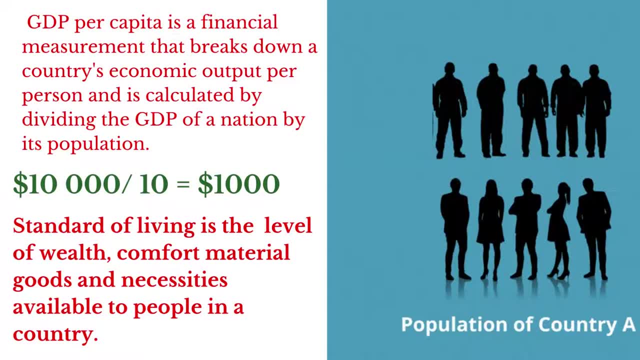 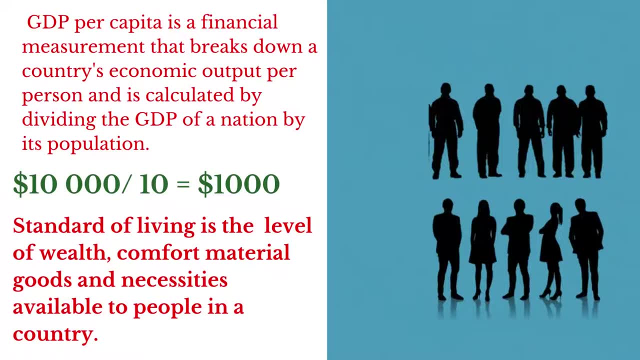 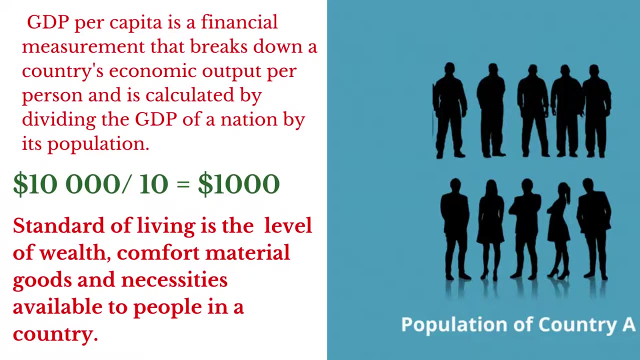 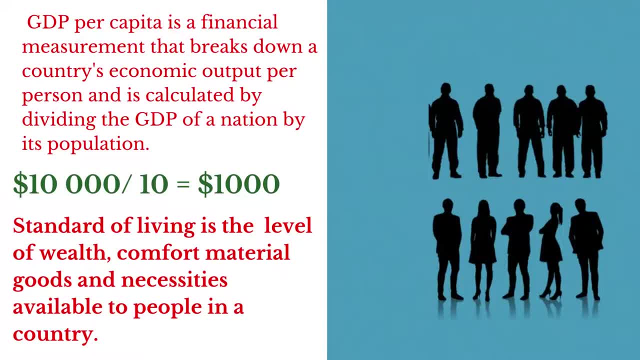 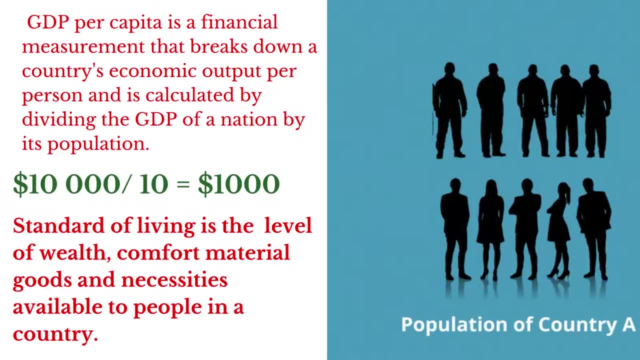 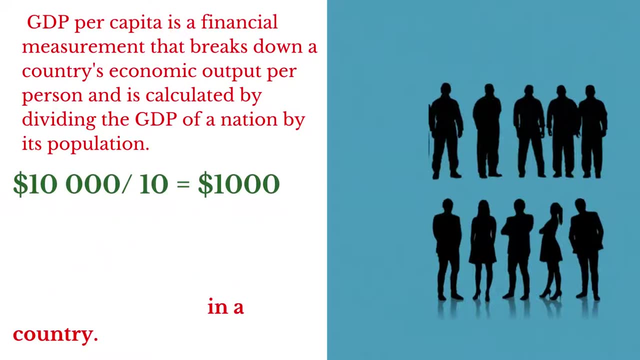 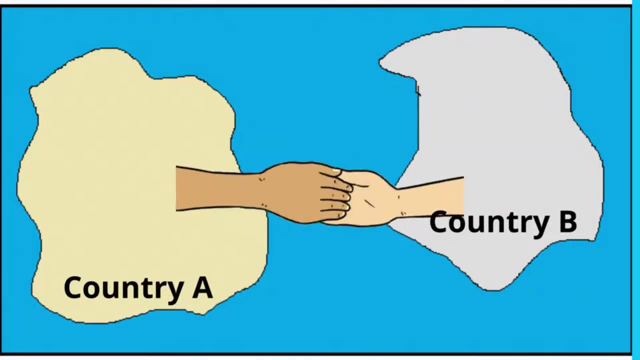 The GDP per capita helps us to determine the standard of living of a country, And when we talk about standard of living, we're talking about the level of wealth, comfort, material goods and necessities available to people in a country. Transactions are not confined to interactions between sellers and buyers only within a country. 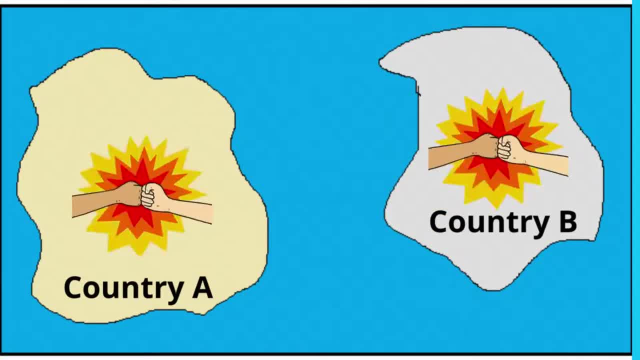 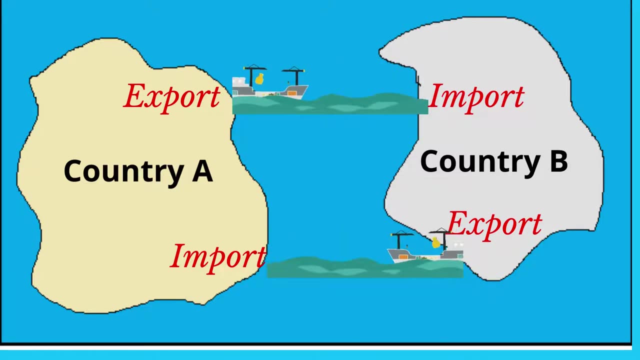 Transactions can be extended to the interactions between buyers and sellers within a country, sellers and buyers between countries as well. When a country sends goods and services to another country for sale, it is known as export. On the other hand, when goods and services are brought, 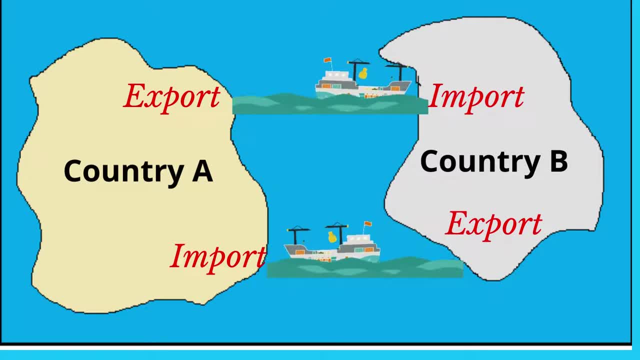 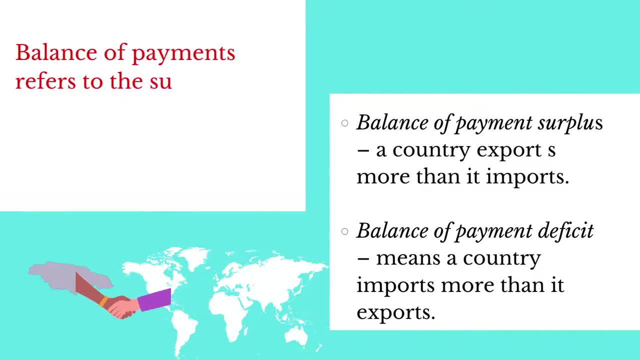 into the country from abroad for sale, it is called import. A summary of all economic transactions between a country and the rest of the world is known as a balance of payment. Under this heading of balance of payment we can talk about balance of payment surplus and. 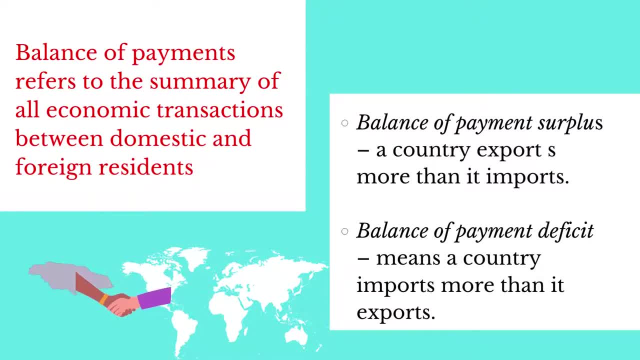 balance of payment deficit. A balance of payment surplus exists when a country exports more goods and services than it imports. This means that the country's earnings are more than the country's earnings. The country's earnings are more than the country's earnings. A balance of payment deficit, on the other hand, exists when a country imports more. 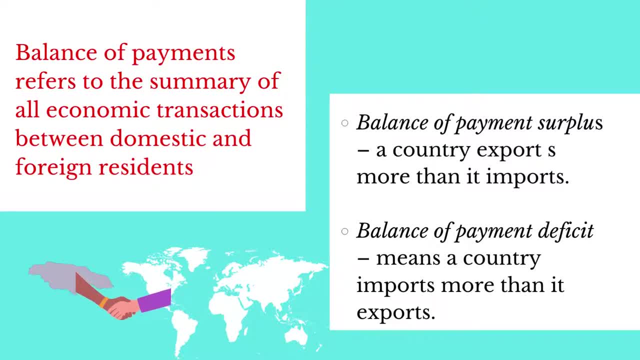 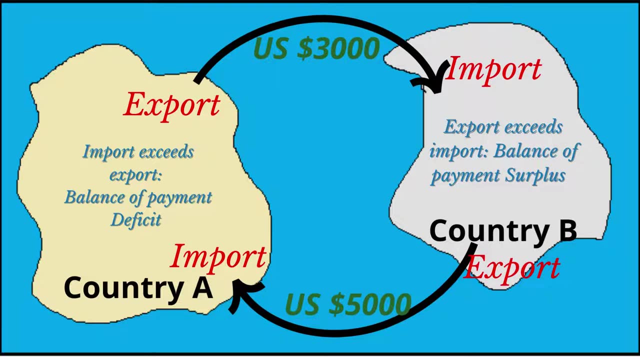 goods and services than it exports. This means that the country is paying out more foreign currency than it is earning. In the illustration, country A has a balance of payment deficit. A balance of payment deficit is a balance of payment surplus. Countries with a balance of payment deficit often. 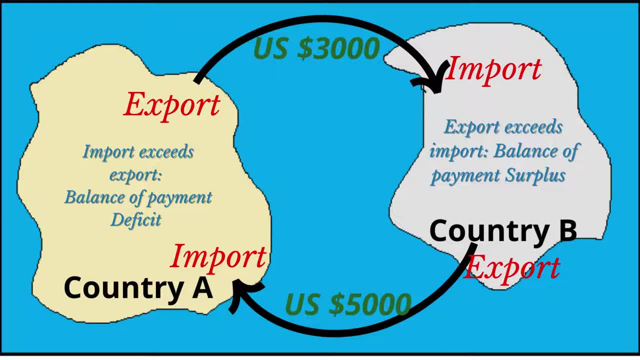 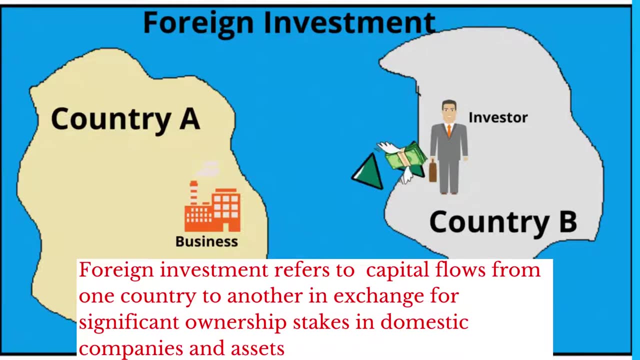 incur a debt burden, which is a large amount of money that one country owes to another and find difficult to pay. A balance of payment deficit is a balance of payment surplus. A balance of payment deficit is a balance of the goods and services that the country spends 왠가. 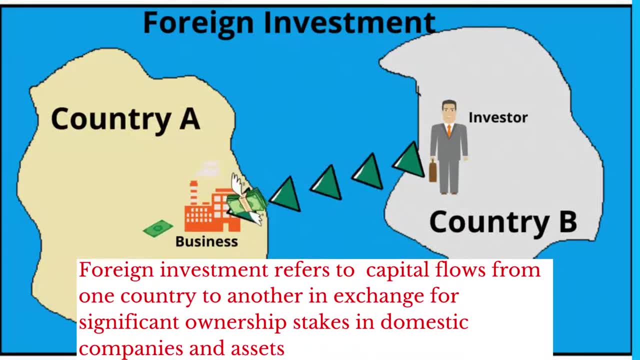 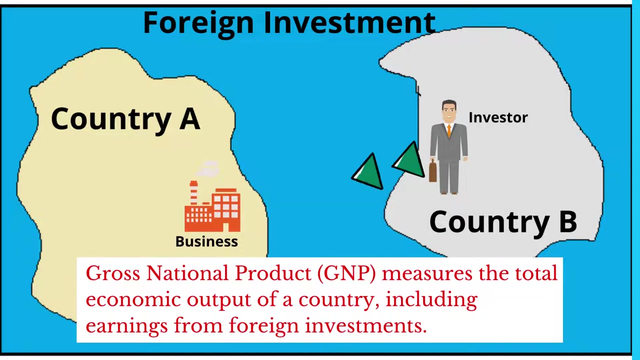 The balance of payment deficit is a lower is Very wealth there. iev. a balance of payment deficit is a more equal balance of payment. the country can help to boost the economy by increasing employment and production. for the source country of the foreign investment, money will be returned. 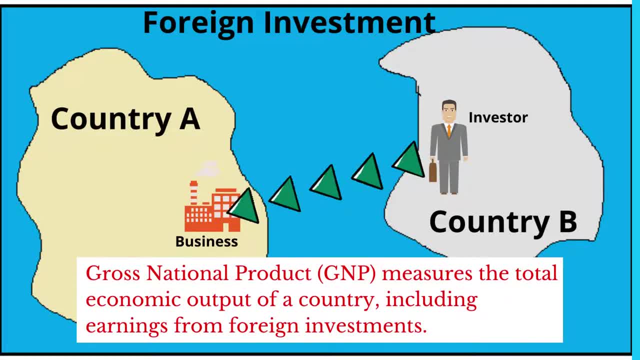 into the economy through the profits from the overseas business. this brings us to another term. you have already been introduced to gross domestic product. now we're going to be talking about gross national product or gnp. the gross national product measures the total economic output of a country, including earnings from foreign investment. 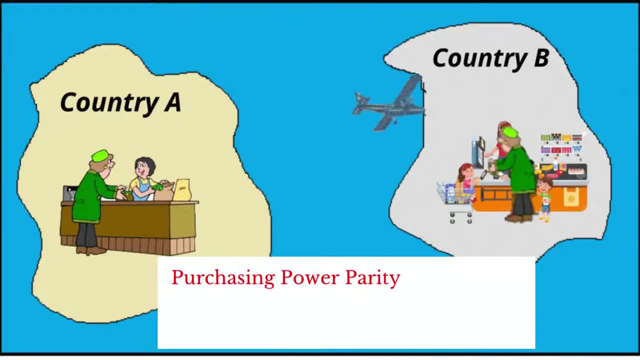 as people migrate to other countries, they find that the ability to pay for goods and services will change. that is, there is a change of the purchasing power from one country to another, so we can talk about purchasing power parity or purchasing power ppp. this refers to how much things would cost if all countries used the same currency. 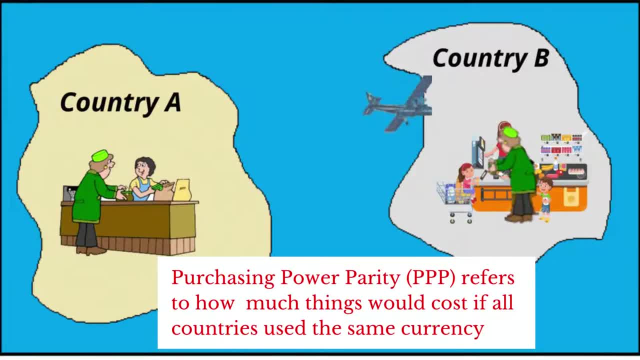 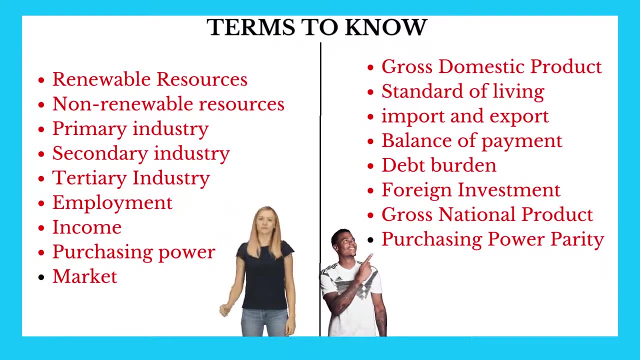 it is the rate at which one currency would need to be exchanged to have the same purchasing power as another currency. so here's a look back at the terms, or at least some of the terms that we've discussed. let's take a few minutes to see how we can apply these terms. 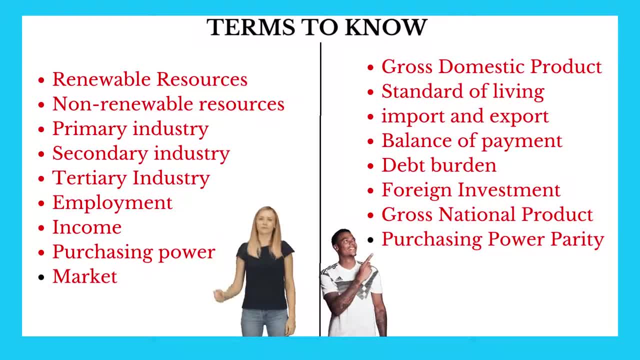 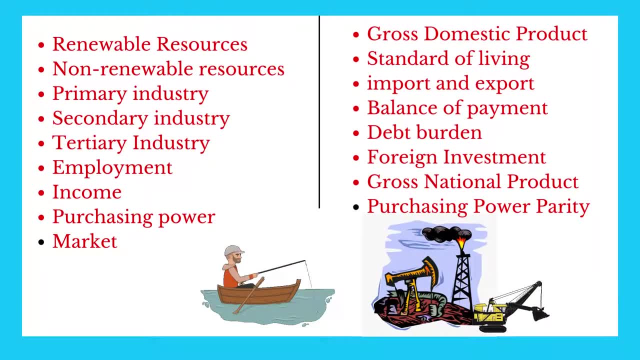 to the industries that we study under the csec syllabus. the csec geography syllabus, that is, the fishing industry of belize is a primary industry focusing on the extraction of renewable energy resources. the oil and natural gas mining industry of trinidad and tobago. 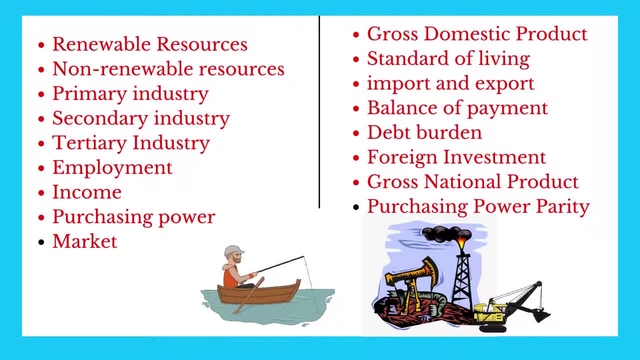 is also a primary industry. however, it focuses on the extraction of non-renewable resources. the oil and natural gas industry of trinidad and tobago is very expensive to operate and therefore one source of its capital is foreign investment investment, The main market for both the products of Belize's fishing industry and the products of 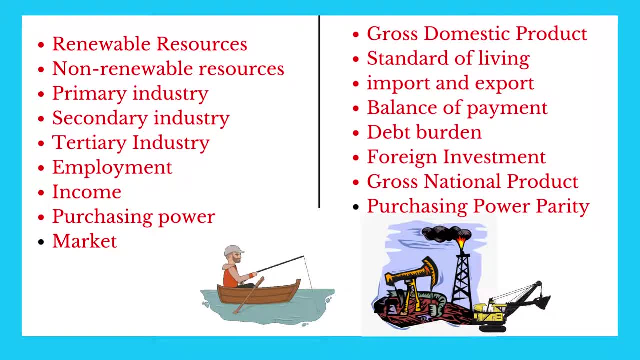 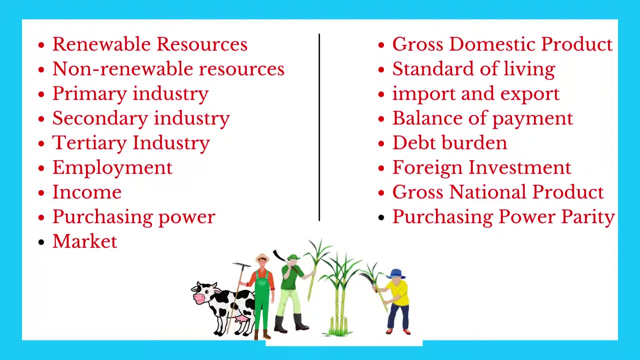 Trinidad and Tobago's oil and natural gas industry is the USA. In the process of exporting these products to the USA, foreign exchange is earned. This money can then be used to pay for goods and services imported into the country. Agriculture in the Caribbean has experienced a lot of changes, For example, the benefits. 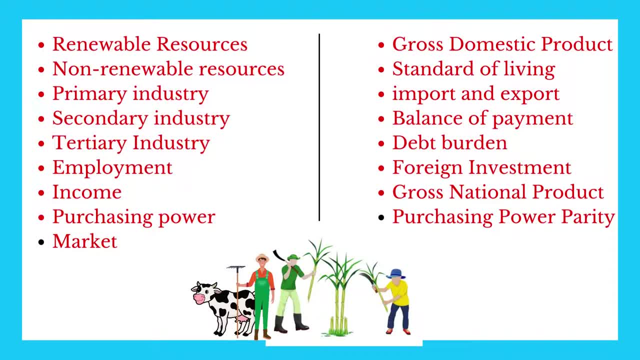 it has received in the past year has been significantly increased. In the past from its European market has largely decreased. As such, many countries in the Caribbean have had to seek other markets. Unfortunately, many Caribbean countries import more food than they export, resulting in a balance of payment deficit and a large debt burden. 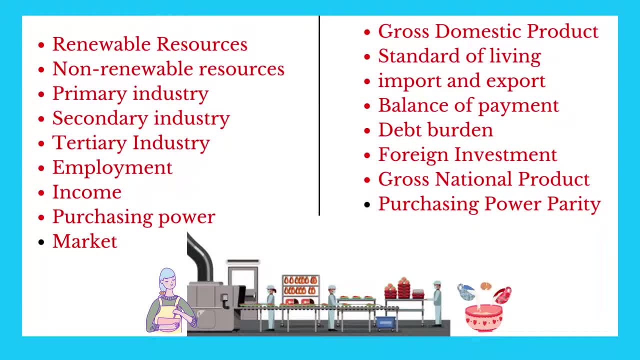 One of the main secondary industries in the Caribbean is the food processing industry. This industry contributes to food security and also provides goods for export. This industry is also one of the main markets for the agricultural goods produced In the Caribbean. food processing industries are: 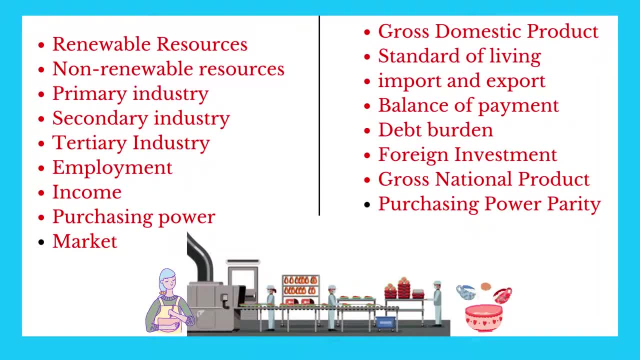 available in many different countries, but they are very limited. The size of food processing industries varies from small to very large. Some of the large food processing industries have overseas branches, and income from these branches contributes to the gross national product, which in most cases means the food that is being grown from a country used by the European countries. 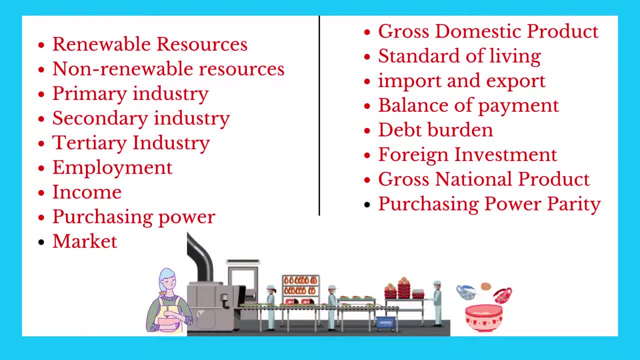 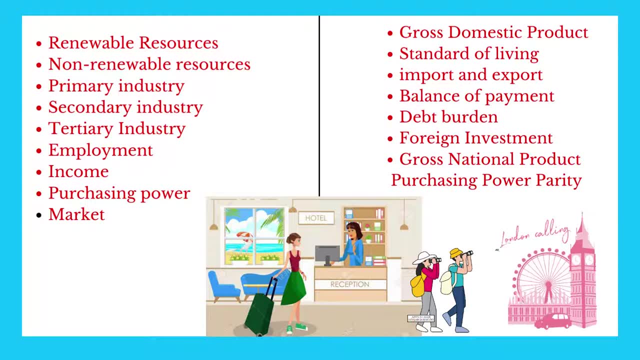 which in turn help to raise the standard of living for the citizens. One of the main tertiary industries in the Caribbean is tourism industry, which provides accommodation and recreational services to both local as well as overseas visitors. The main tourist markets are North America and Europe, which are accessible to the Caribbean. 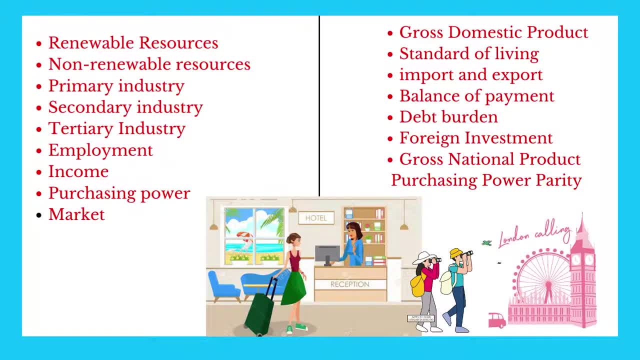 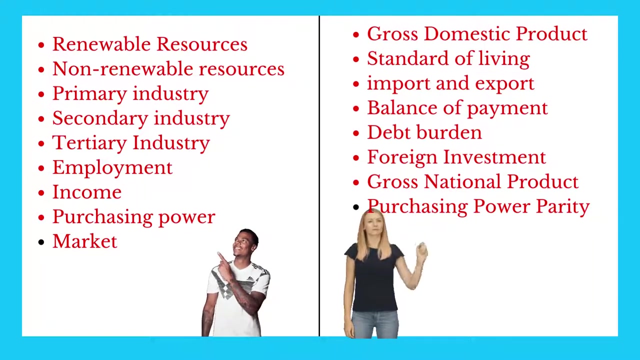 The industry provides employment to locals, who receive an income for offering exceptional services to the visitors. This income increases the purchasing power of the employees. For most Caribbean countries, tourism tourism- is the largest contributor to the gross domestic product. Okay, so I hope that this was useful to you. 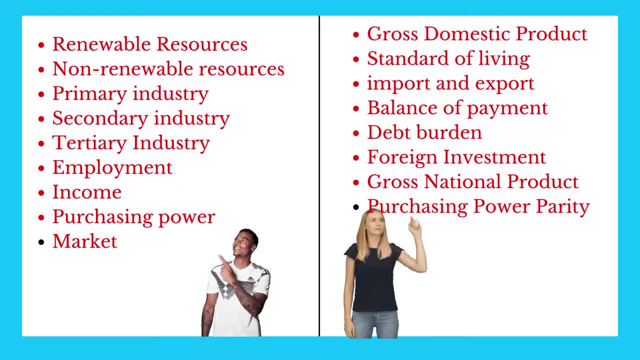 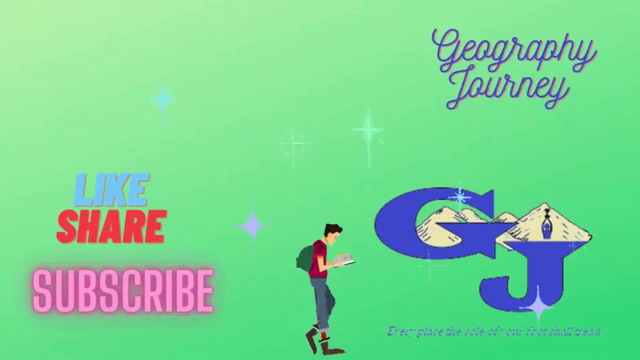 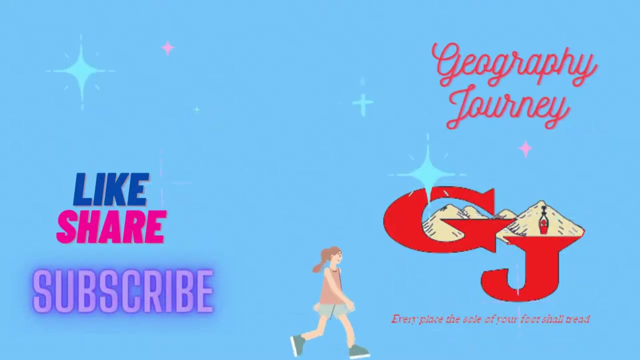 Now it's time for you to find some past paper questions and practice using these terms. Once again, I want to thank you very much for your continued support. If you have not yet subscribed, please go ahead and do so, And don't forget to like this video and to share it with somebody else.